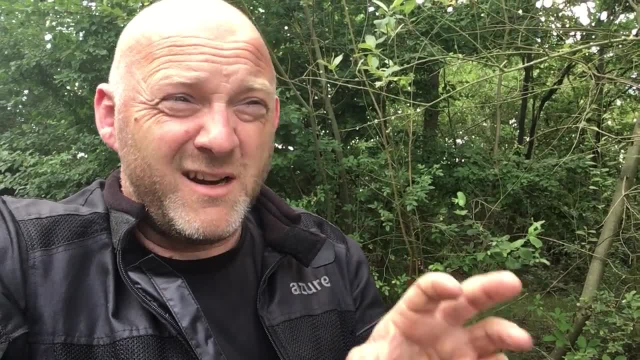 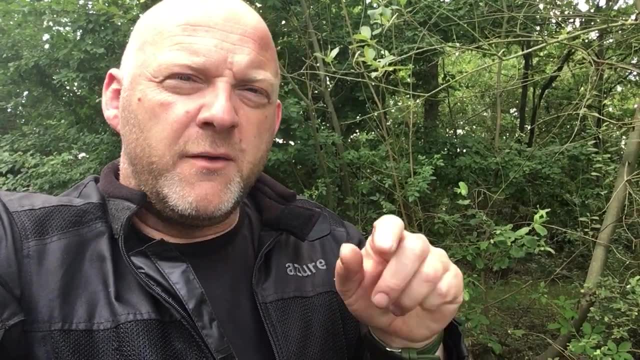 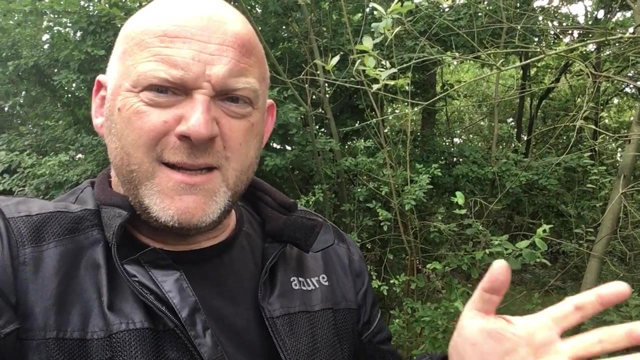 road tyres and I was just about doing about 50 miles to the gallon and I was getting on a full tank of fuel about 200 miles as well. Now, the last few months, especially on a different set of tyres- I'm on the Anarchy Wild, which are more the off road type, and it started off at about mid 40s miles per gallon, and now it's crept up to 50 and 55. Today on the out leg, when I was doing more back roads, I was actually on 58.6 miles per gallon, which is really odd. 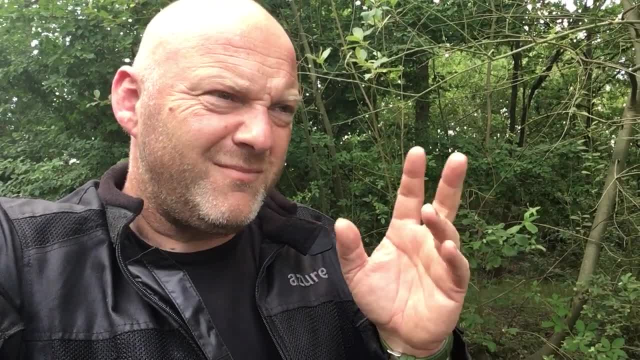 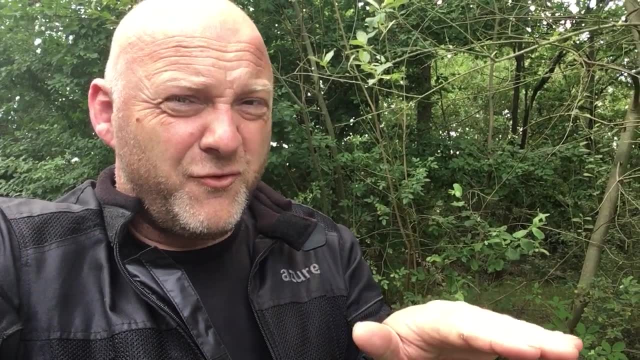 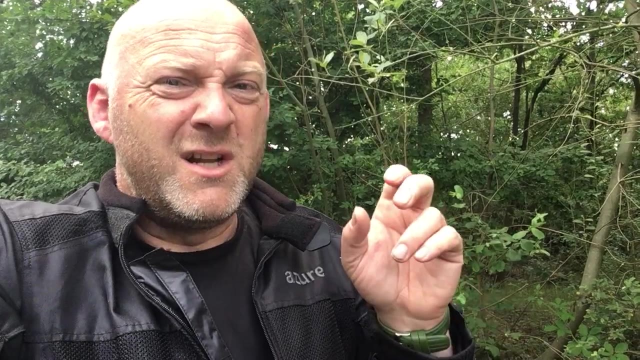 Now, a lot of this is down to do with aerodynamics, Air pressure and temperature. you know your air density and also your weight elevations. I've been riding sort of flat terrain, really gentle climbs. I've been operating mostly about 300 feet above sea level, apart from where one bit I went up to about 800 feet. 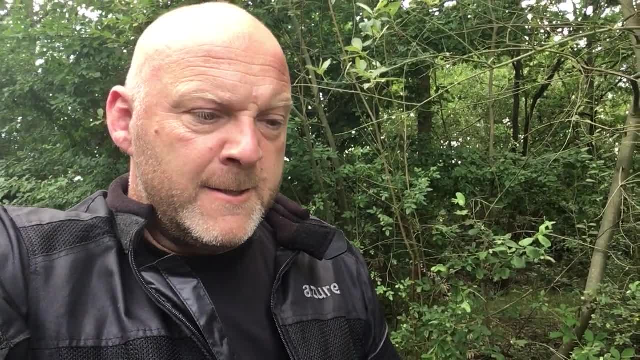 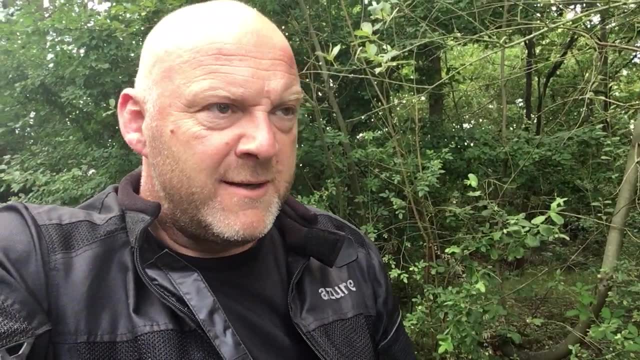 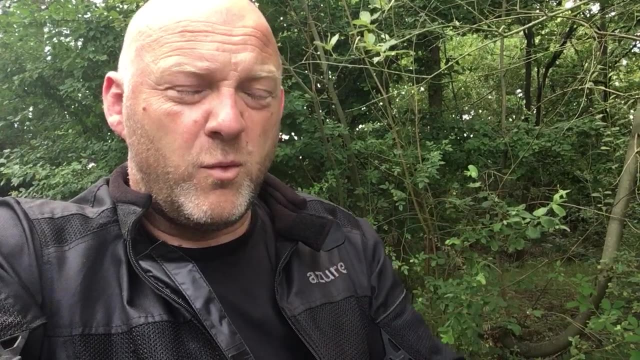 above sea level for about 15 miles. that's about it. So not grand, not really big elevation changes either. It's been a kind of a steady 23,, 24 degrees today. I actually crept at about 25 at one. 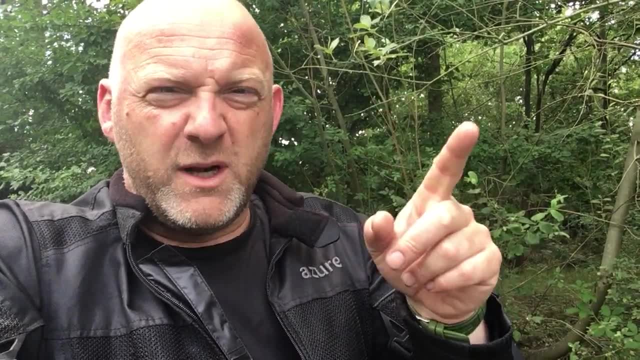 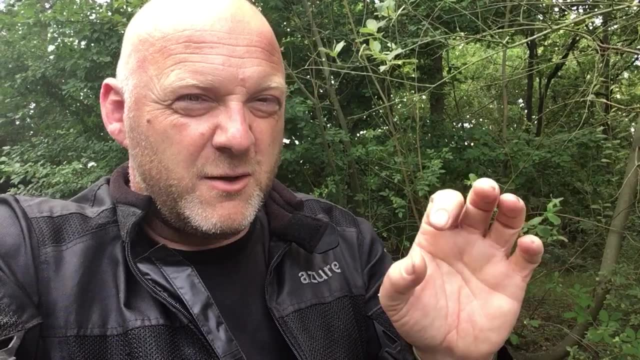 point I noticed on my out leg. I was at about 24, 25 degrees and the air seemed a little bit thinner. It might not be, but it seemed a little bit thinner On the way back. temperature dropped down to about 23 at one stage and it seemed a little bit thicker as well. A little bit. 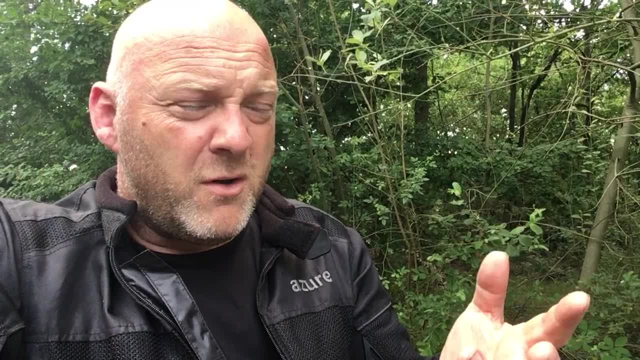 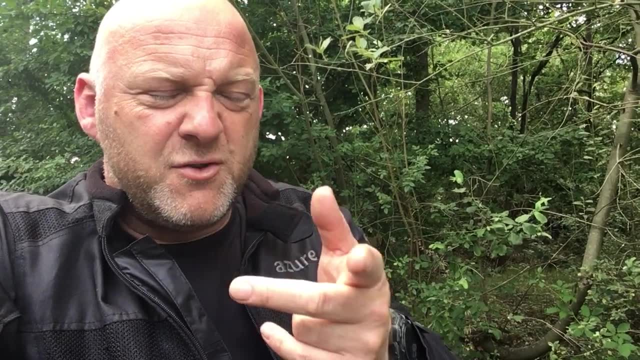 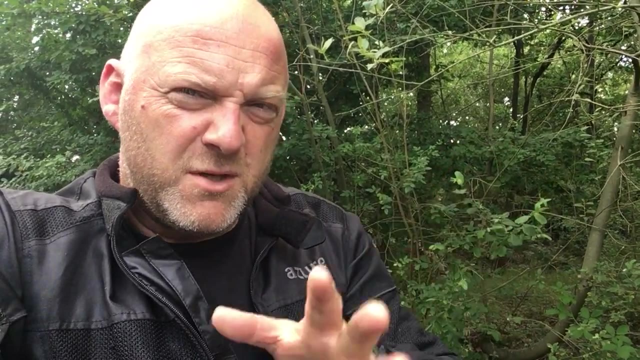 of extra wind resistance. I'm not sure if that's relevant or not, but on the way out I was getting better mileage, On the way back I was getting less. so that's an interesting thing. But one of the big things is obviously tyre wear. Now I've noticed, obviously since my 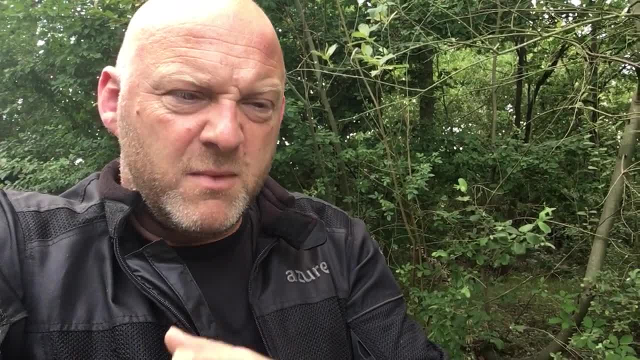 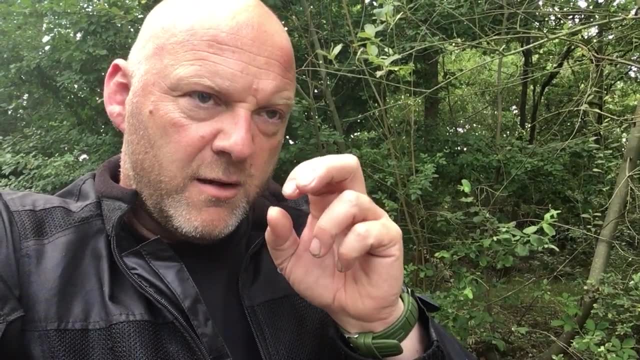 tyre's been wearing down, that I'm getting better mileage. but also it depends on your tyre pressure, of course, and I tend to run my tyres a little bit, a couple of psi more, and I know that's on the road- That'll give me better tyre wear. 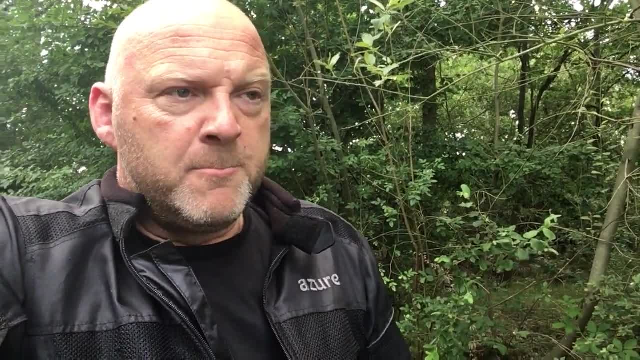 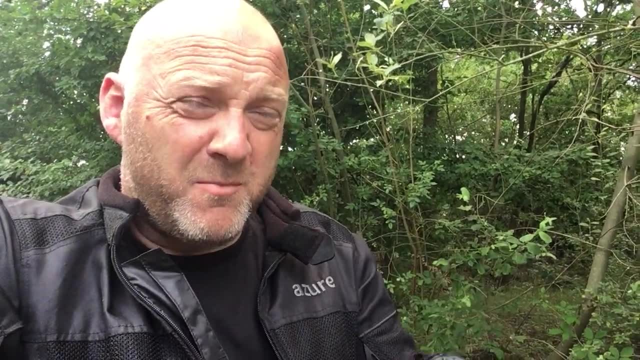 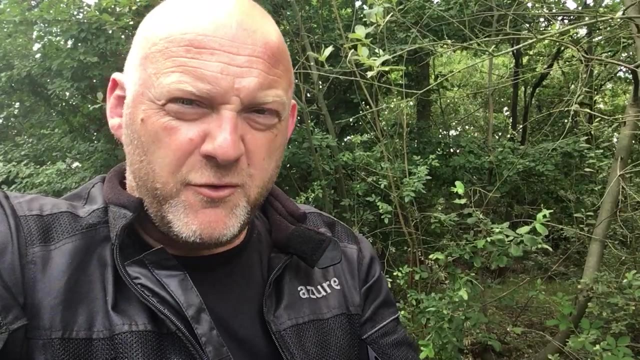 and better mileage as well. but it's just just changed this big fluctuation, so i'm really not sure what's caused it. uh, but i know, when i first got the bike i was getting about, say, 50 miles to the gallon and i was also getting about 200 miles on a full tank. now i'm saying getting well over 50. but 50, let's say 53, 55, uh, today 58 at one point, uh, and i'm getting about 230 miles to the tank. i think if it was actually went down to you know fumes, there's nothing in it. i think this tank would get about 250 miles, which is really impressive. so i'm just wondering you: 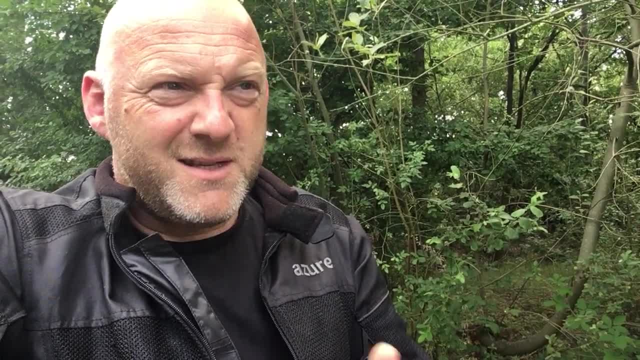 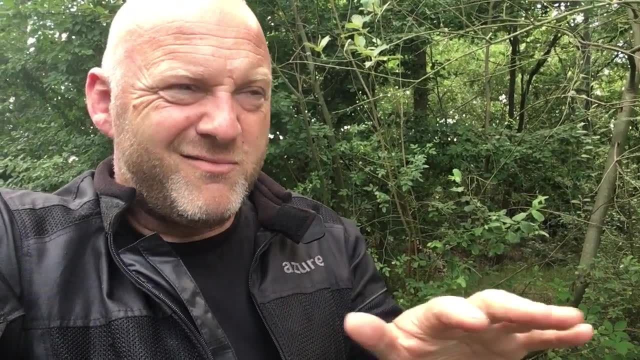 know, i put it out to you guys. what do you think this is, you know, causing it? is it just tires? is it you know the? you know the atmospheric pressure and everything like that, which you can think it's been constant, so i can't really say it's massive changes there, so it's got to be down to the tire. 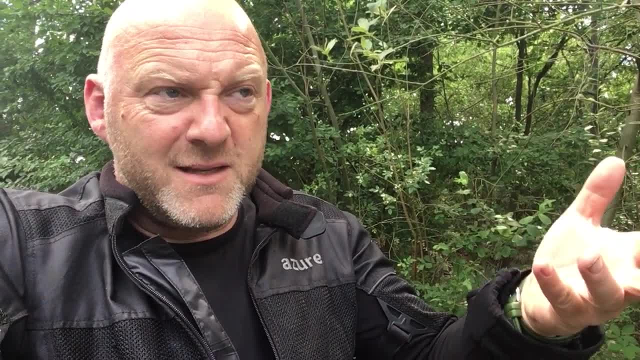 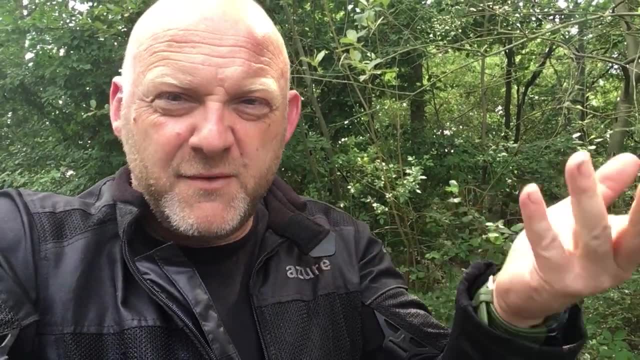 wear. i think the more the the more your tires wear down and, let's say, the correct operating pressure, the better mileage you're going to get. possibly- i don't know, maybe you need you know. if there's an expert out there, let us know. anyway, i just thought it was weird very. 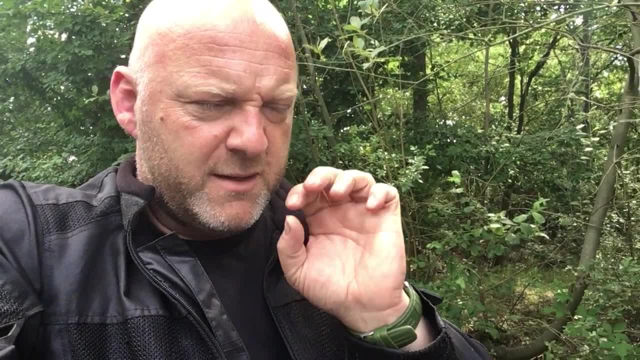 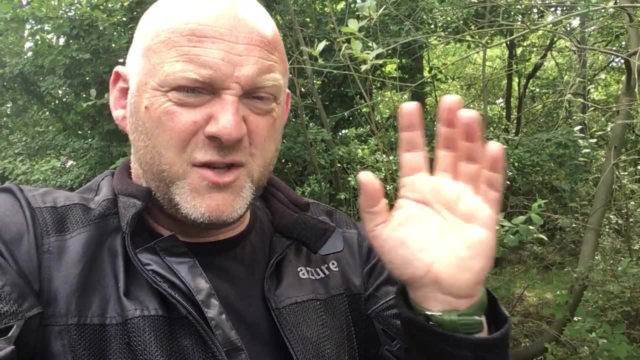 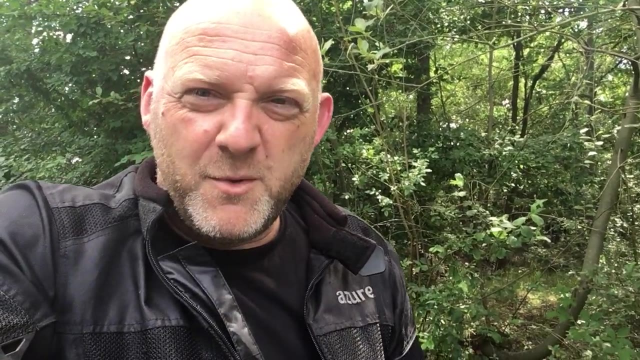 weird tire, uh, not a very weird. uh you know fuel consumption today on the bike. let's say it seems to get really uh great mileage and then it dripped down to, but still really better than it's ever been. go figure, right. well, hope you uh found that as weird as i did, because i still 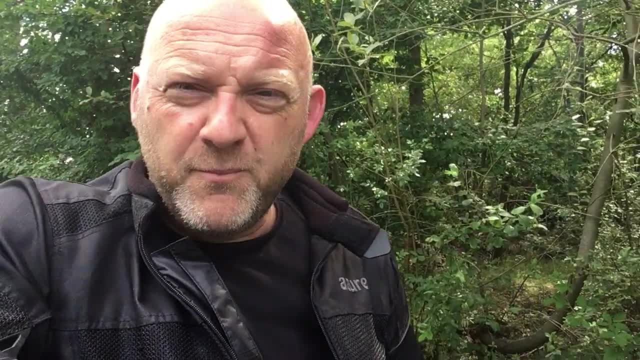 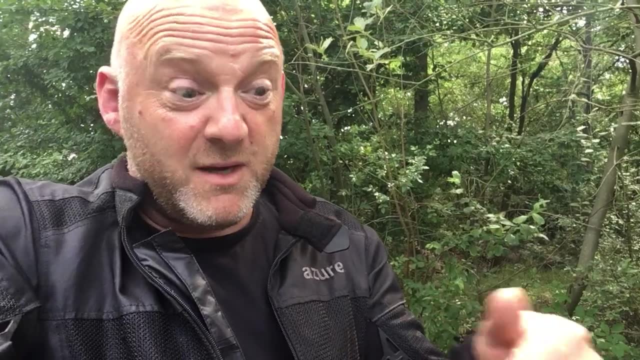 can't work it out. you know i'm getting a headache just thinking about it. right, anyway, uh, tomorrow i'll get the new bike. so you know, all those have been a faithful servant and it's been brilliant mileage. obviously, uh, it's gotta go right. catch you on the next video, whenever that is uh subscribe. 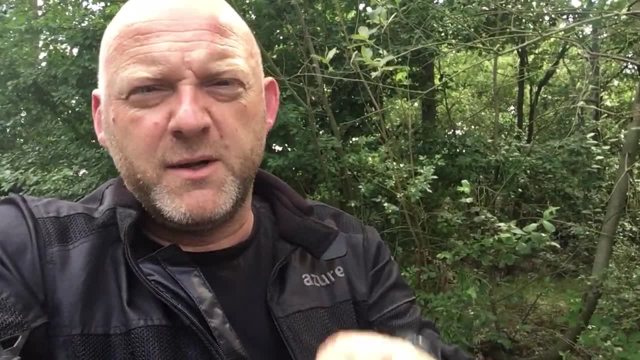 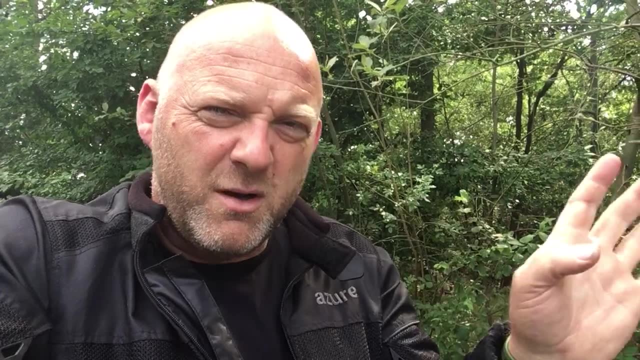 and all that good stuff, notifications, bow, leave loads of comments as well. let me know what you think. uh and uh, check out the website revelatorcom. all the support pages are there, all the links are there, all the podcast links and everything like that, and uh, well, what's left to say? but catch you on the next video. 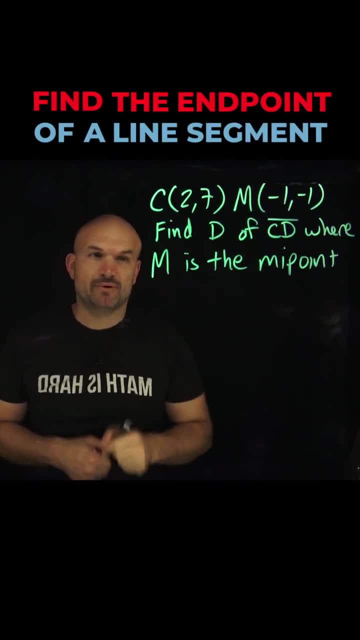 In this video it says: find d of cd where m is going to be the midpoint. So we don't know what d is. However, we do know that m is going to be the midpoint of those two values. So the important thing we need to understand is just use your midpoint formula. We know. 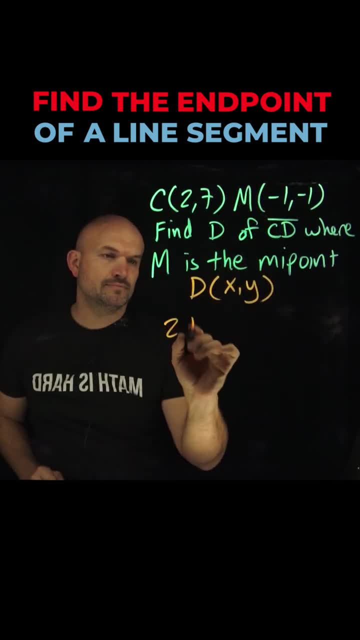 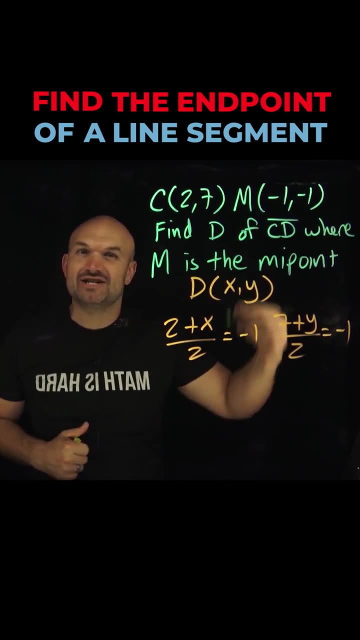 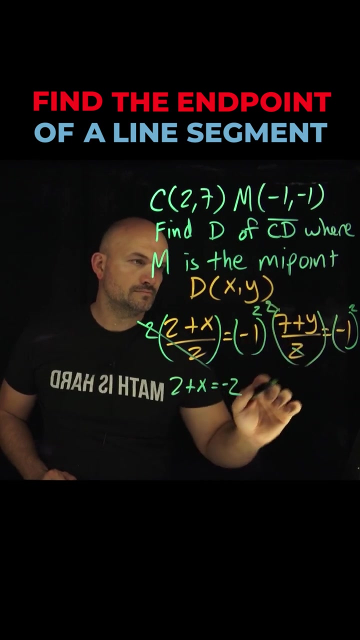 2 plus x divided by 2, is equal to a negative 1.. We also know that 7 plus y divided by 2 is equal to also a negative 1.. Now all we simply need to do is use our inverse operations to solve for an x and solve for a y. Now we have found the other endpoint. when given one,